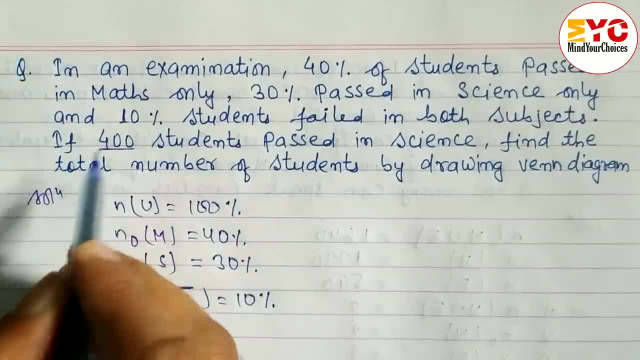 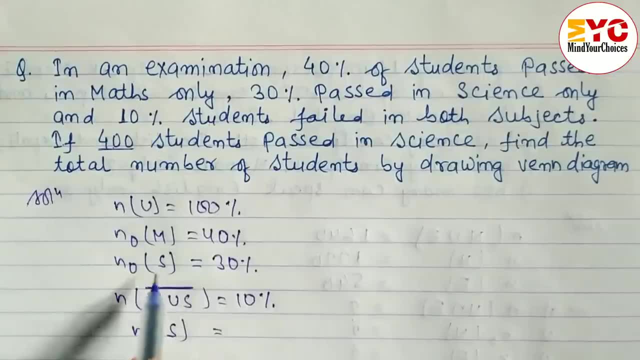 Again, here you can see one number is given here: 400.. If 400 students passed in science, it means NS only is not given, Here only is given. So only we have to write. But what is here If 400? 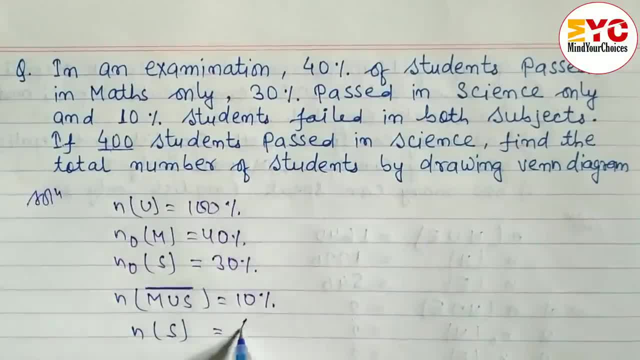 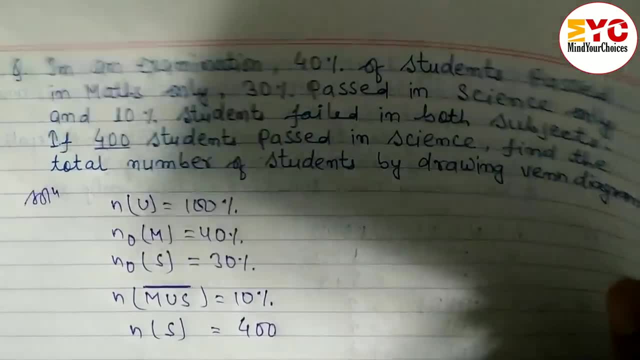 students passed in science. So NS is equal to 400.. And what we have to find out? Find the total number of students by drawing. We have to find out total number of students. Okay, now one thing you have to keep in your 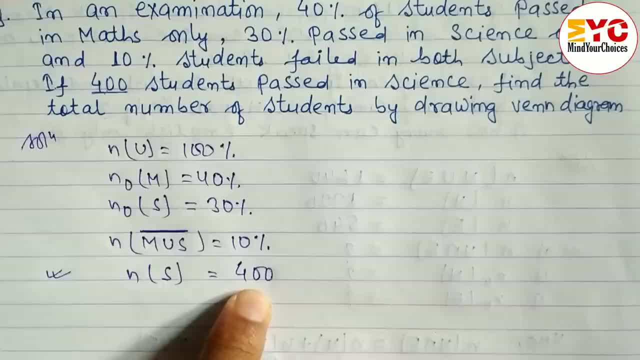 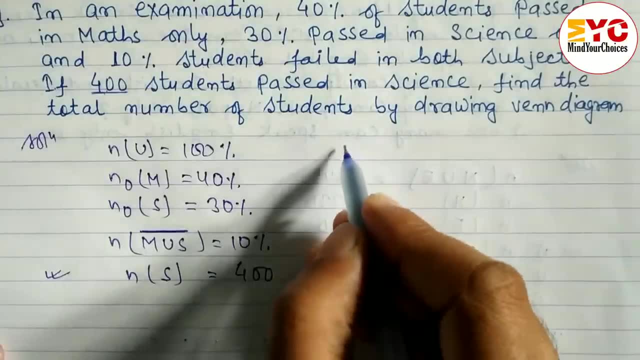 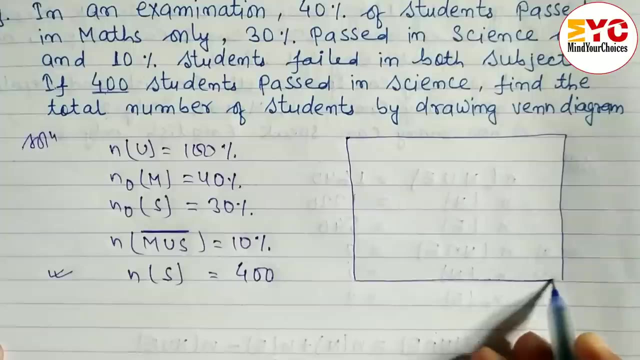 mind This question: NS is given in number. we have to find out NS in the form of percentage. Okay, here, by drawing a Venn diagram, let's draw the Venn diagram, First of all. we can use formula also. but question is there: by drawing a Venn diagram, then let's use the. 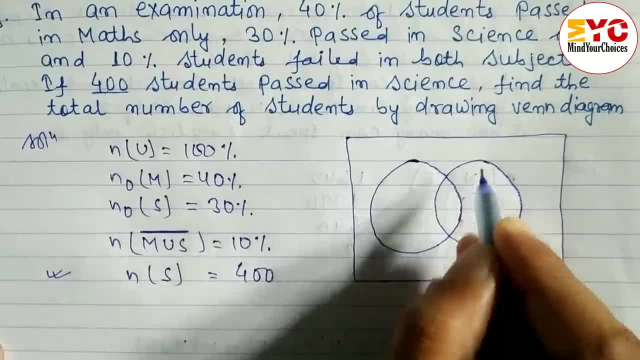 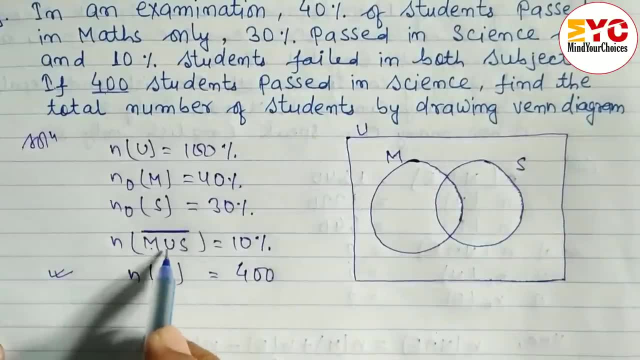 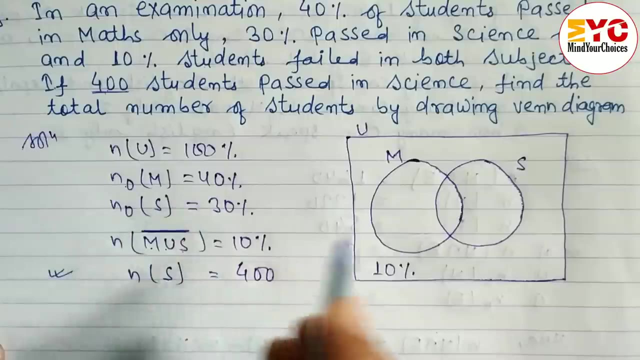 Venn diagram And find out the answer. This one for math and this one for science. And here we have to write down U, here M, union as complement means outside of set. we have to write here 10%, Here only M 40%, So here we have to write on 40% only as 30%, So we have to write: 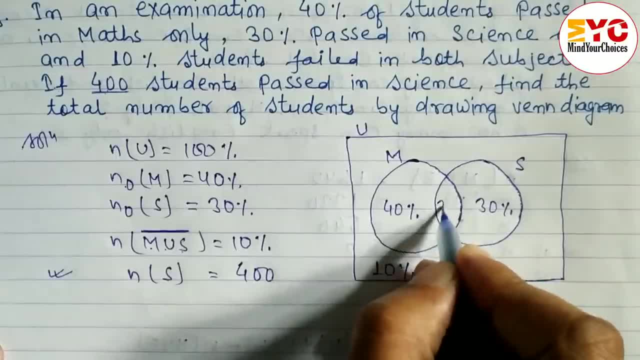 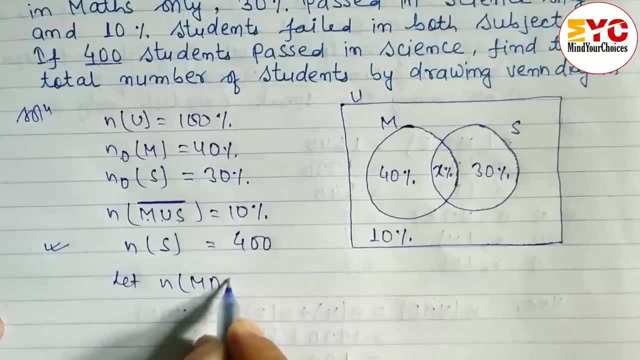 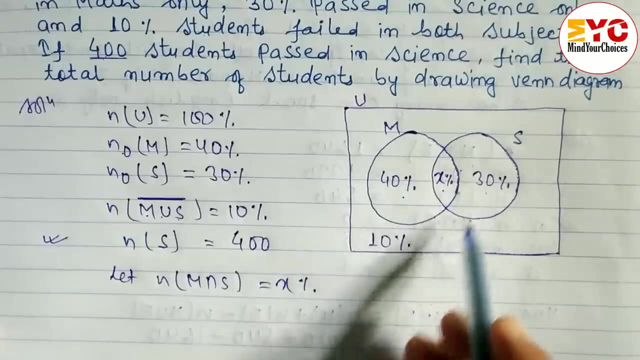 here 30% Intersection is not given, So let here x percent, this one is x, So we can write here And M intersection as is equal to x percent. Okay, up to here. After this, when you add this, all what we get total: 40 plus x plus 30 plus 10 is equal to: we get total total. 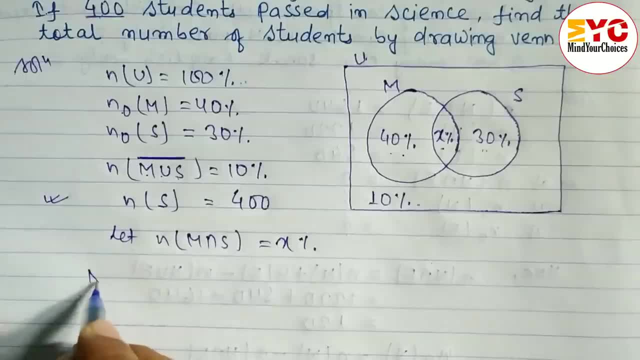 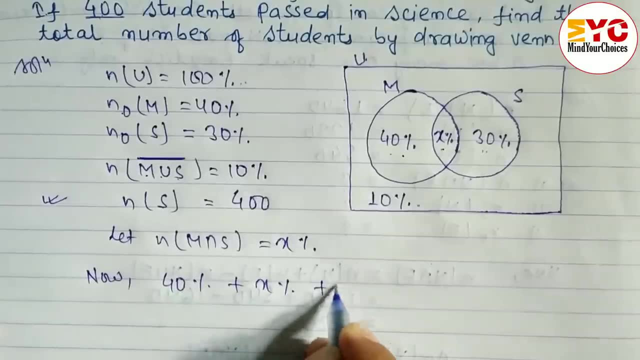 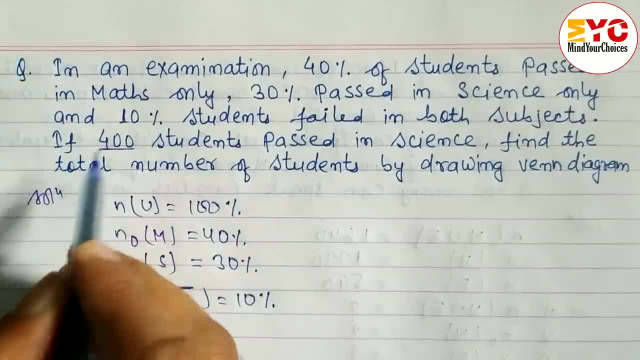 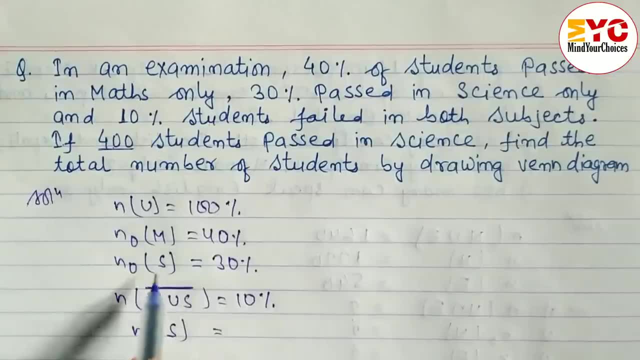 Again, here you can see one number is given here: 400.. If 400 students passed in science, it means NS only is not given, Here only is given. So only we have to write. But what is here If 400? 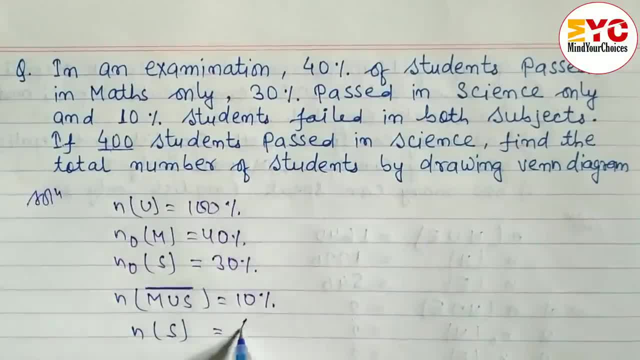 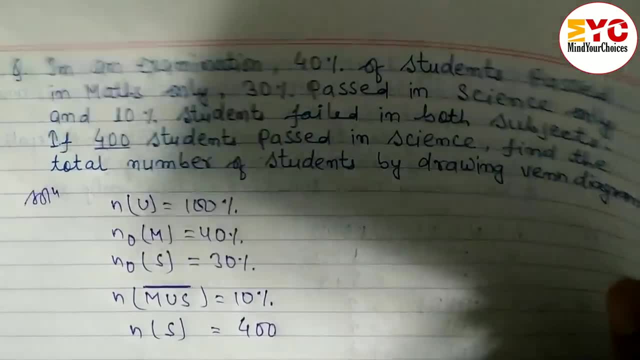 students passed in science. So NS is equal to 400.. And what we have to find out? Find the total number of students by drawing. We have to find out total number of students. Okay, now one thing you have to keep in your 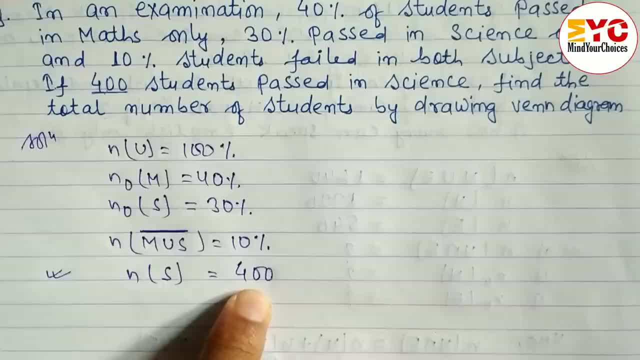 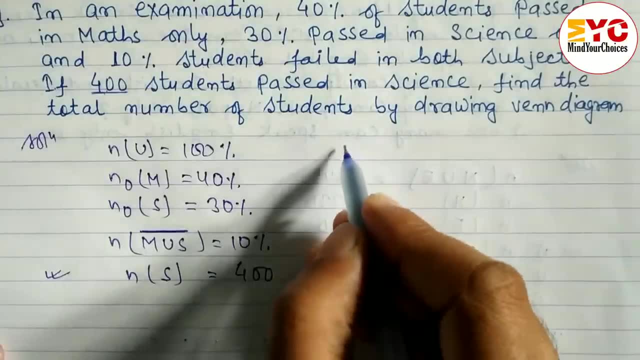 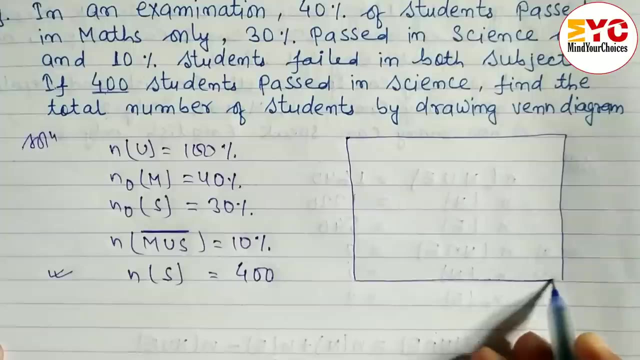 mind This question: NS is given in number. we have to find out NS in the form of percentage. Okay, here, by drawing a Venn diagram, let's draw the Venn diagram, First of all. we can use formula also. but question is there: by drawing a Venn diagram, then let's use the. 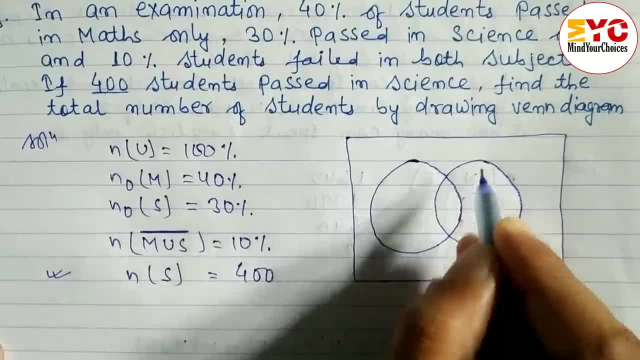 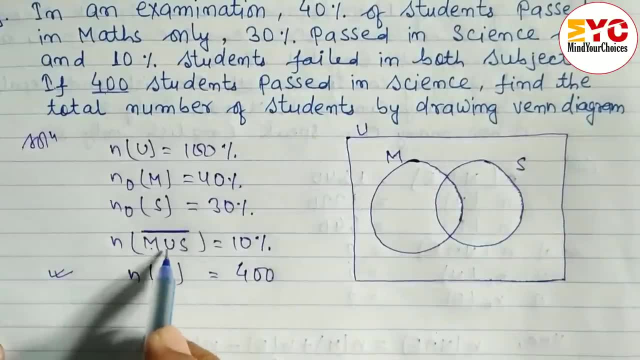 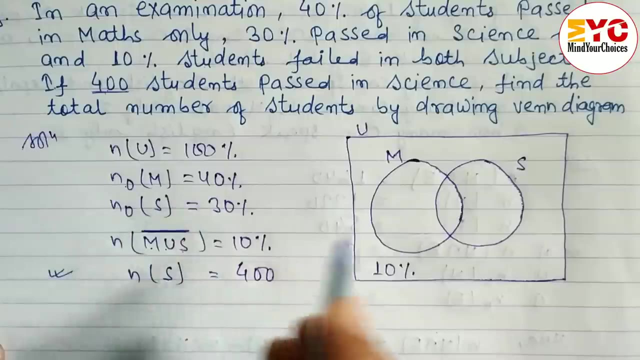 Venn diagram And find out the answer. This one for math and this one for science. And here we have to write down U, here M, union as complement means outside of set. we have to write here 10%, Here only M 40%, So here we have to write on 40% only as 30%, So we have to write: 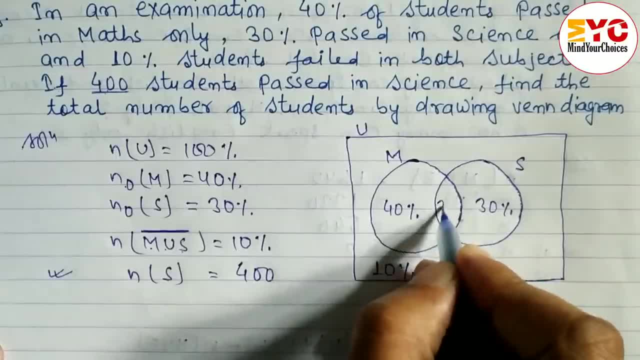 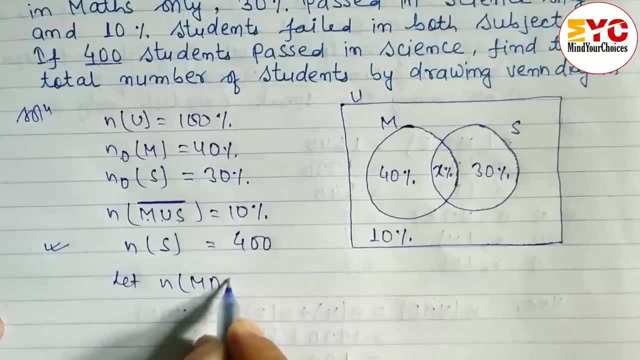 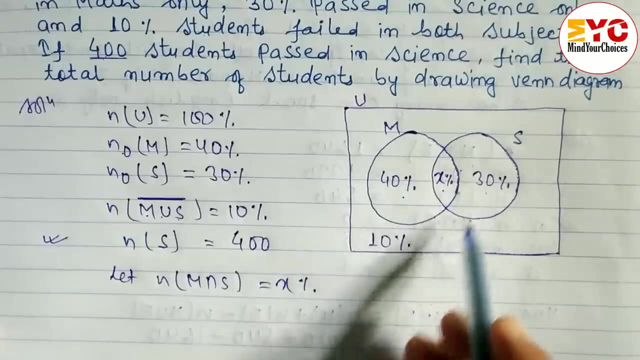 here 30% Intersection is not given, So let here x percent, this one is x, So we can write here And M intersection as is equal to x percent. Okay, up to here. After this, when you add this, all what we get total: 40 plus x plus 30 plus 10 is equal to: we get total total. 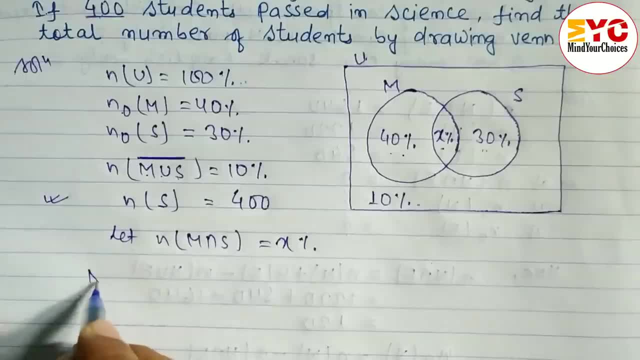 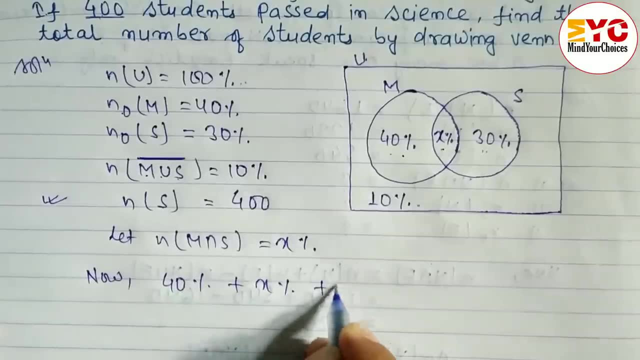 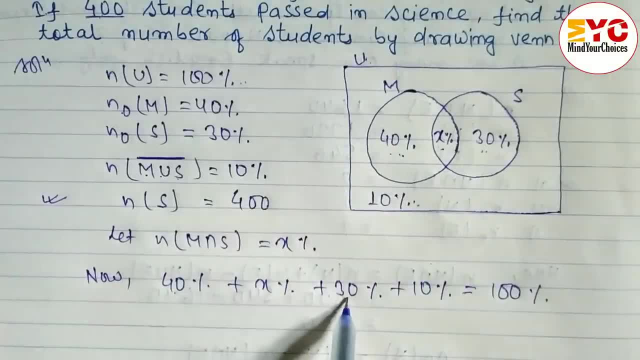 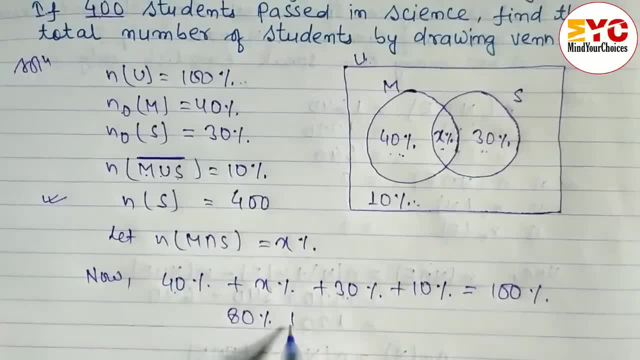 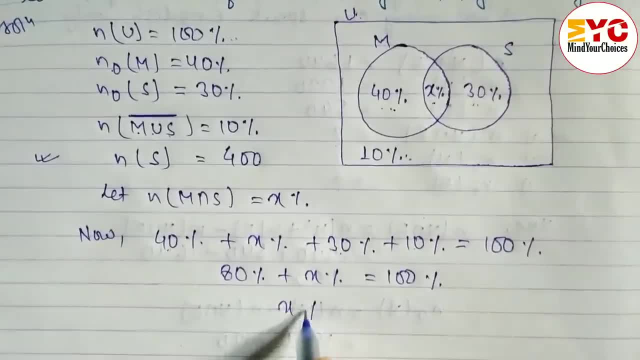 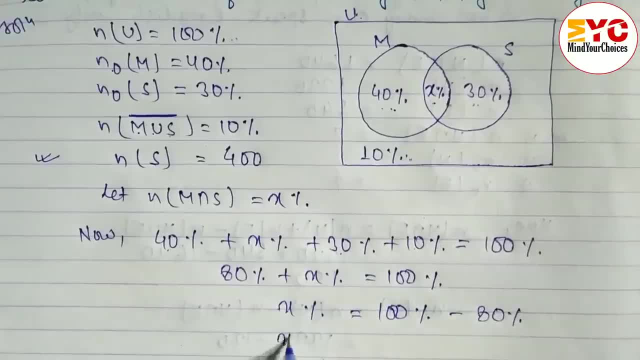 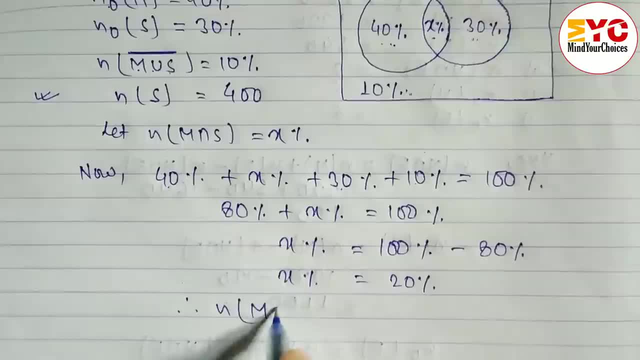 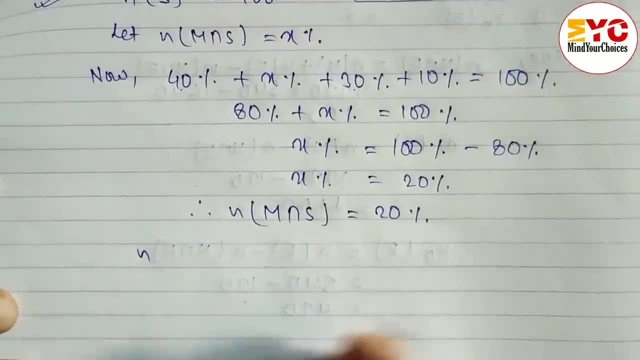 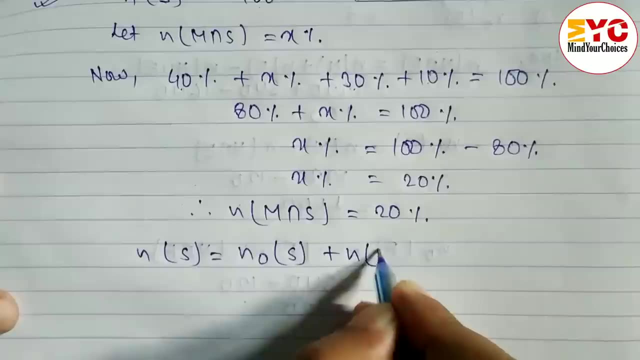 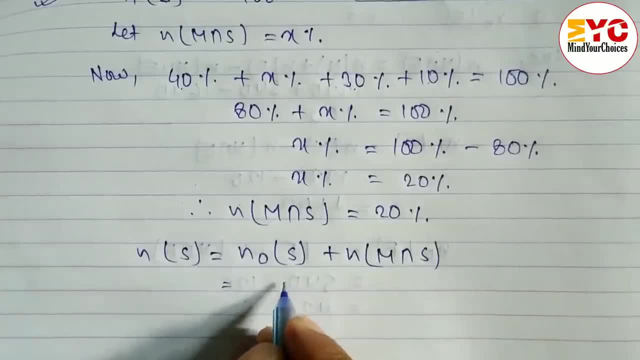 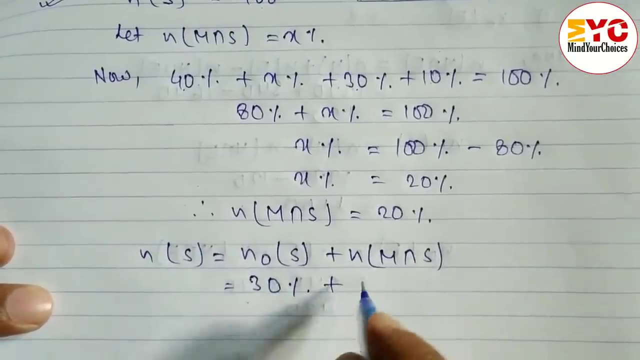 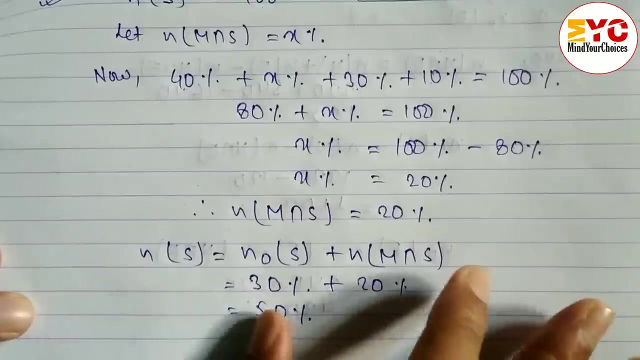 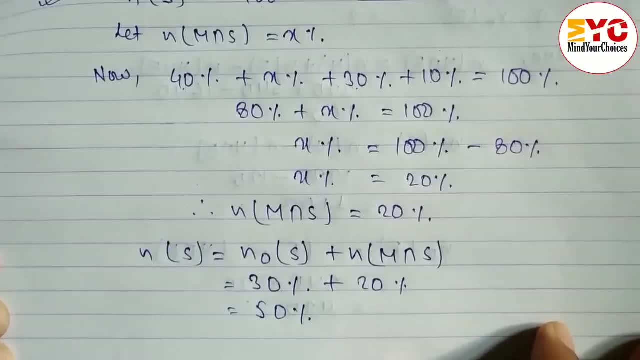 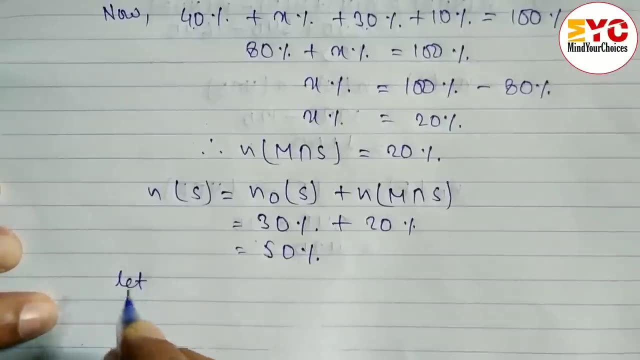 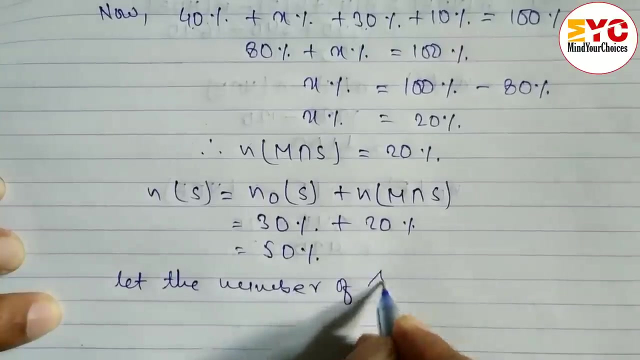 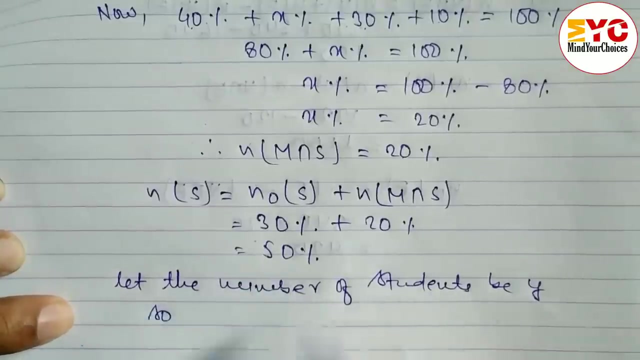 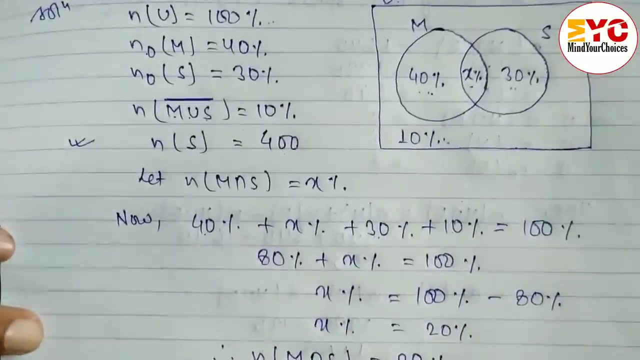 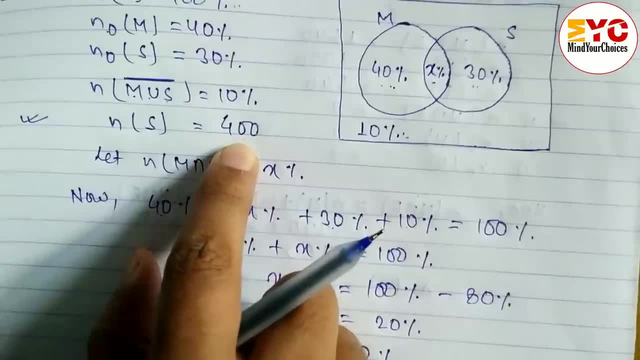 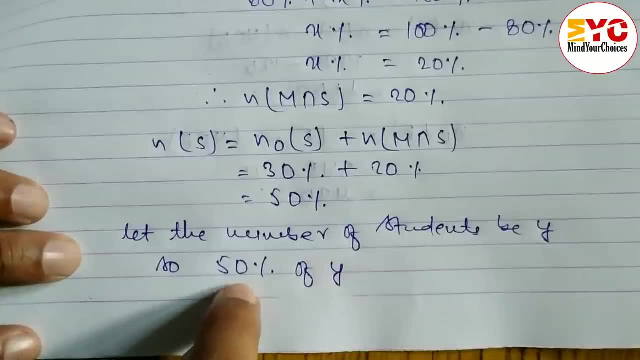 total student is equal to how much 400. 400 is trained passed and here 50% passed is same thing. this 50% passed off of what 50% passed off total number of yesterday is equal to how much 400. now, when you calculate we get total number. 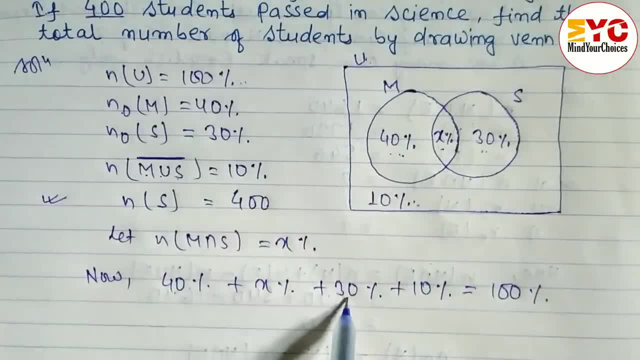 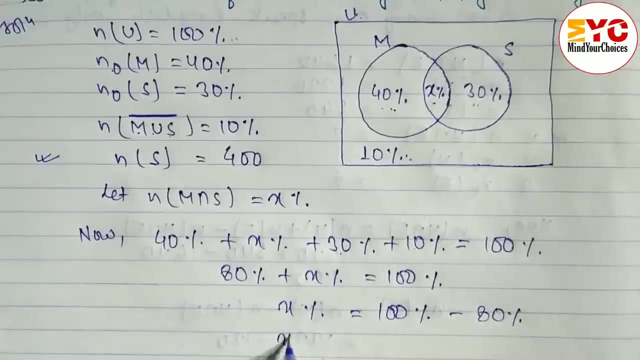 this is equal to: we get total 40 plus 30, we get 70 plus 10, 80, so 80 percent plus x percent is equal to 100 percent. so we get here: x percent is equal to 100 percent minus 80 percent. therefore x percent. 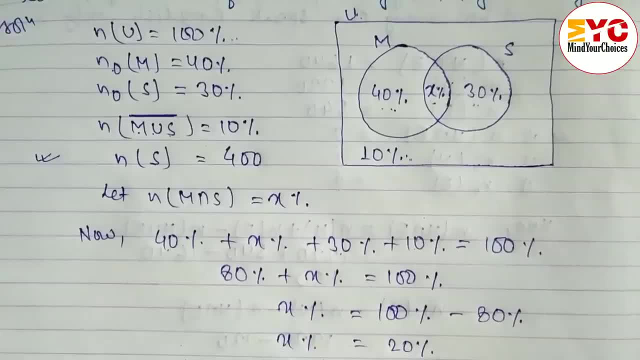 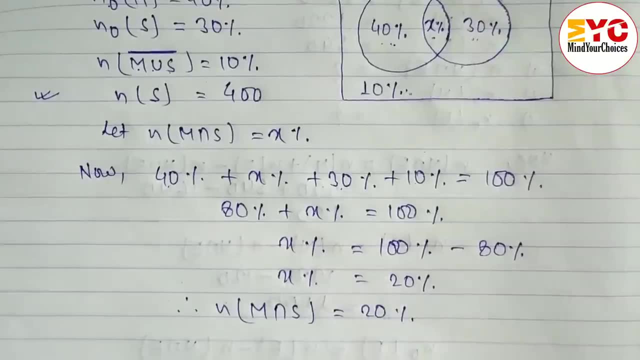 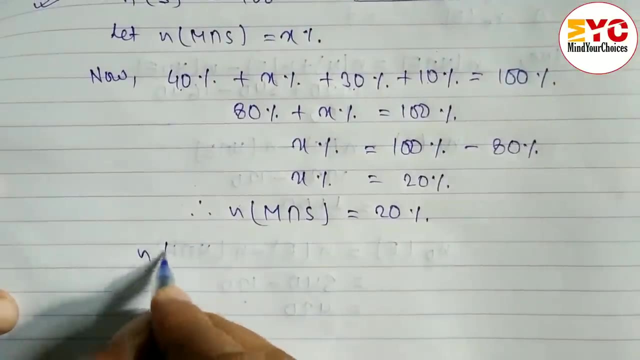 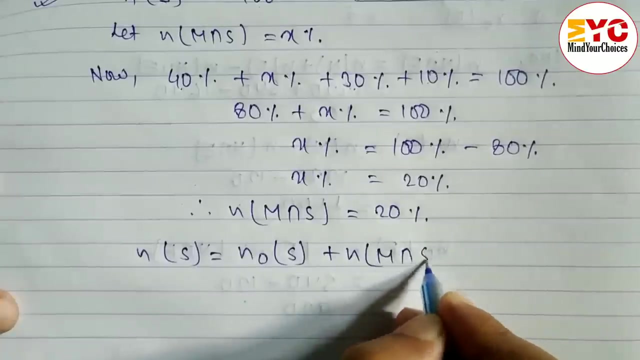 is equal to, we get 20 percent. therefore x percent means which one intersection. so we can write here: m intersection s is equal to 20 percent. now in question, in number, what is given ns? then we have to find out ns in percentage. so to find out ns we have a formula: n only s plus n, m intersection s. 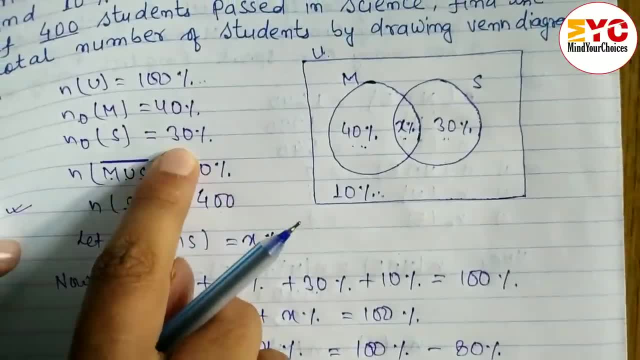 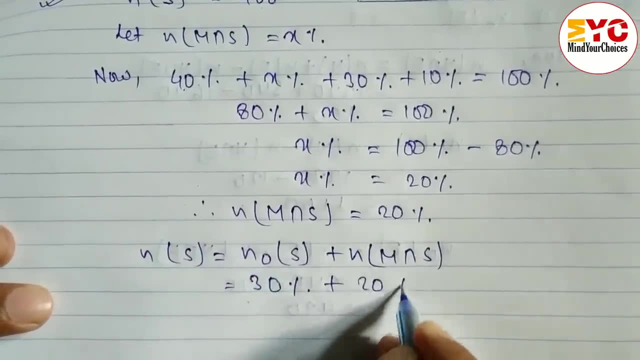 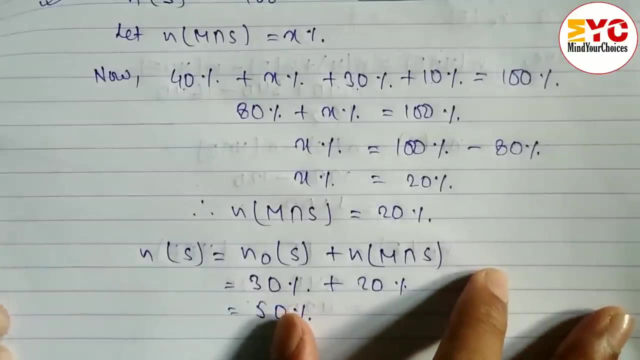 n. only s is given here 30 percent, so we have to write here 30 percent plus this m intersection s, we found here 20 percent. 20 percent equal to 50 percent. if you don't know any formula, if you have any confusion in formula, please you can visit on my formula playlist and you can watch. 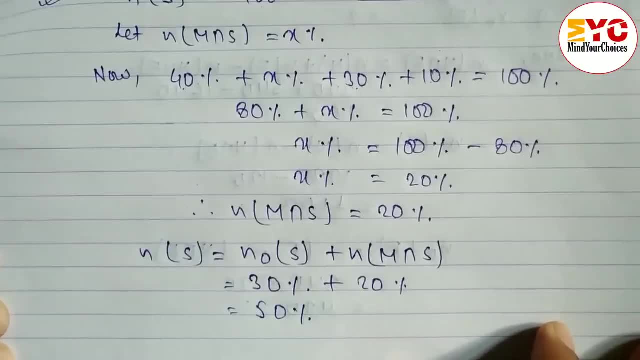 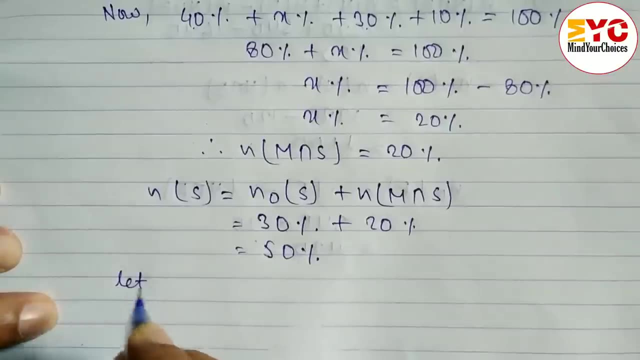 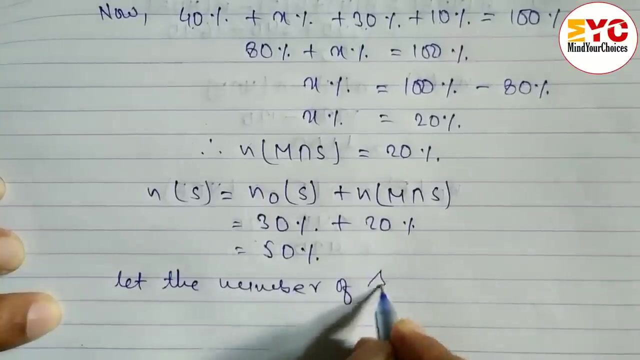 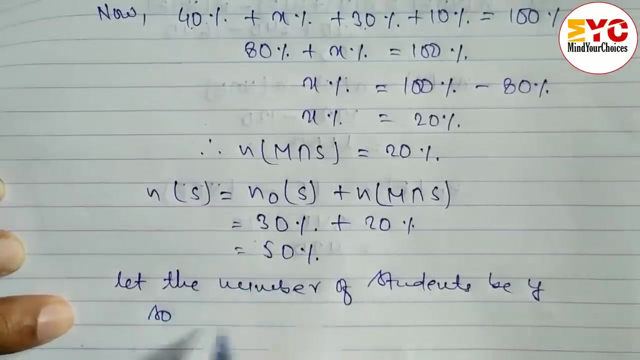 complete formula of different exercise and if you need any kind of formula of any exercise you can comment to now, and this is equal to this. now we have to find out total number of student. let the number of students be Y. so this 50% of Y, 50 percent of why 50% is today in passed in science and 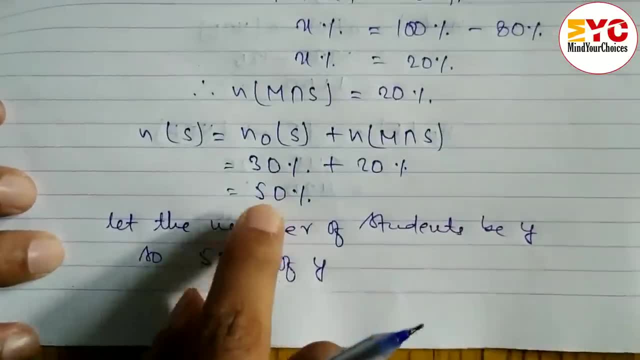 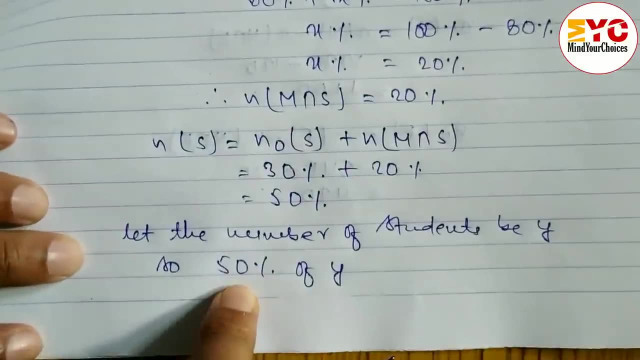 how many number is trained. passed 400, it means this 50% of total student is equal to how much 400. 400 is 20 passed and O here 50% passed. it's same thing. this 50% passed of what 50% passed off. total number of yesterday. 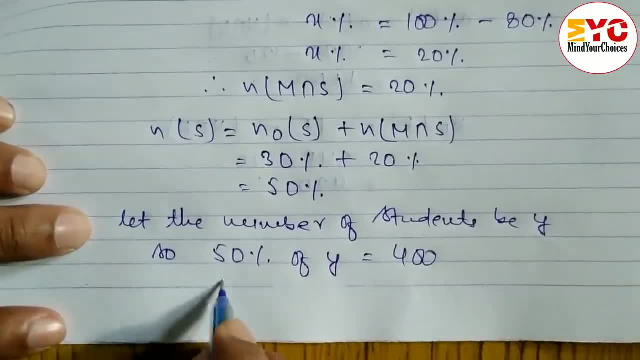 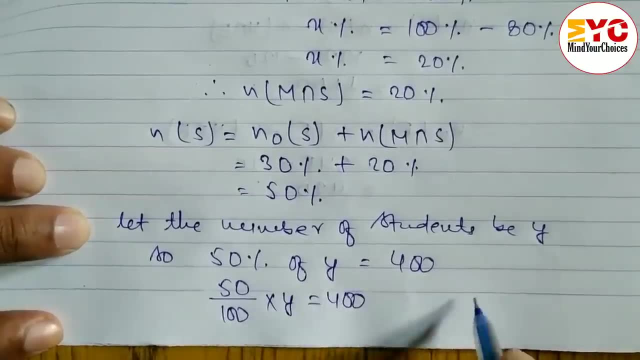 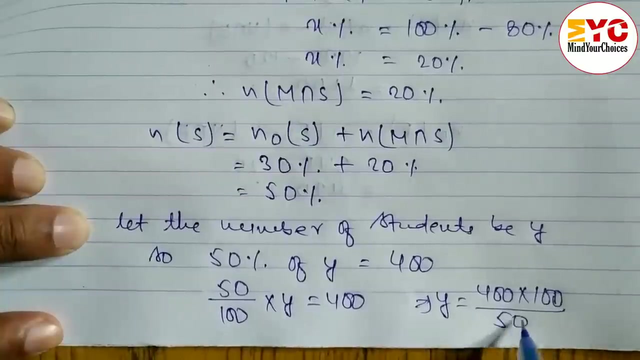 is equal to how much 400? now, when you calculate, we get total number of student from here, 50 by 100 into Y is equal to 400. after this, Y is equal to 400 into 100 by 50. 50 ones of 52, sir. therefore. 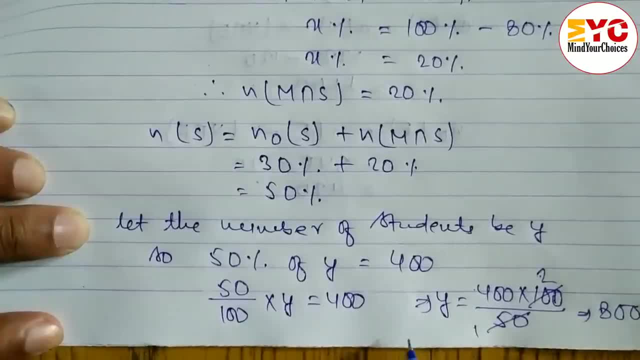 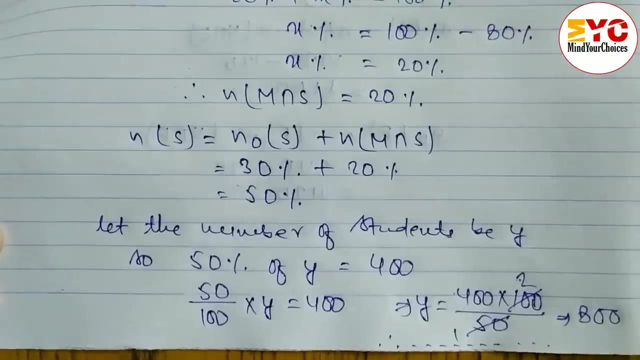 four, twos are eight, eight hundred. therefore, at last, we have to write down. therefore, total number of student is 800. you can write on them at last. total number of strain is 800. if you understand this video, please hit the like button and if you are new on my channel, please subscribe and.